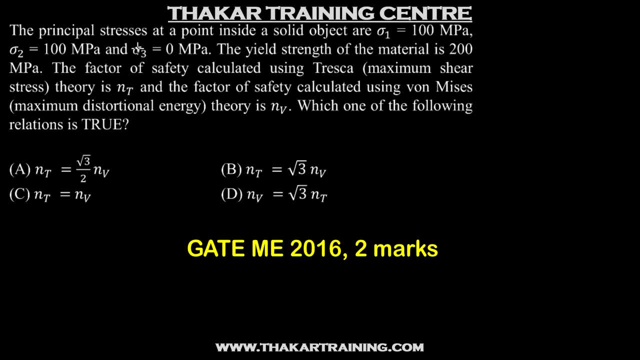 In this question. the principal stresses at a point inside a solid object are given to us. The yield strength of the material is 200 MPa, The factor of safety calculated using Tresca theory is Nt and the factor of safety calculated using Von Mises theory is Nv. Then 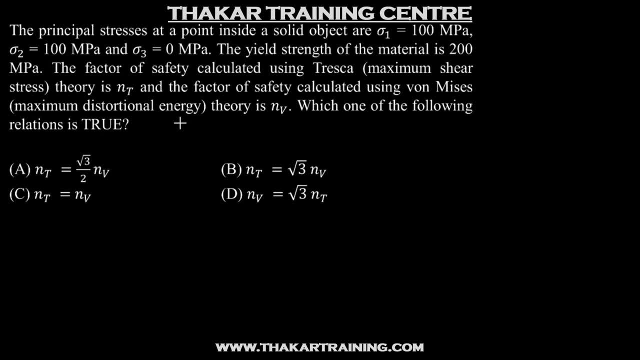 which one of the following relations is true. So let's find out the factor of safety for the two theories. Now we know: for Tresca theory, the equation is: tau max will be sigma y and sigma 2 by 2 fs, where fs is the factor of safety. and for Von Mises theory, the equation: 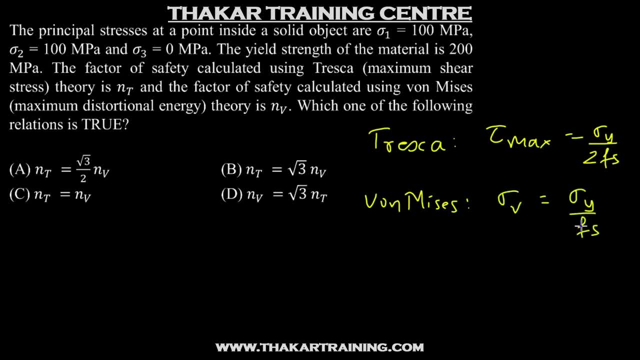 is sigma Von Mises is sigma y by fs. fs is the factor of safety. So how do we find out tau max? when sigma 1, sigma 2 and sigma 3 are known, We have. tau max is maximum of sigma 1 minus sigma 2 by 2, sigma 2 minus sigma 3 by 2.. 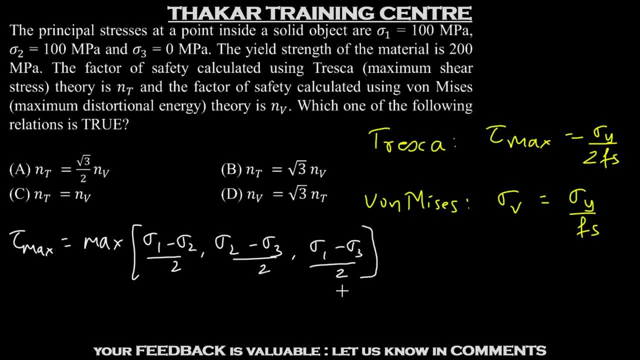 And sigma 1 minus sigma 3 by 2.. So now substituting the values we'll get. So sigma 1 and sigma 2 are equal, So first one is 0.. Sigma 2 is 100, sigma 3 is 0. So this will be 50.. And 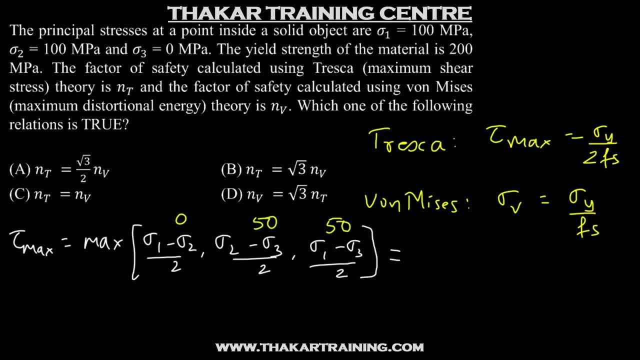 sigma 1 is 100, sigma 3 is 0. So this will also be 50. So the maximum shear stress is 50 MPa, And so Nt, that is the factor of safety, using Tresca theory, will be. So fs goes to. 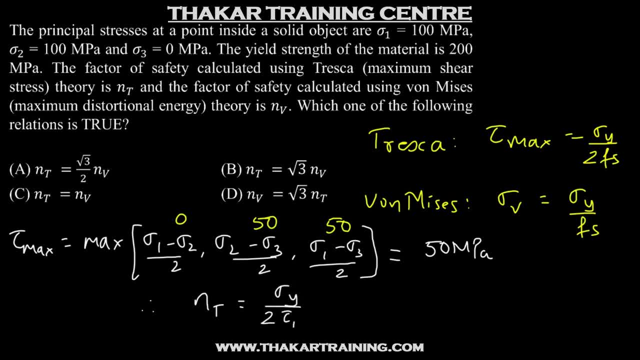 the numerator. This will be sigma y by 2 tau max. So this is going to be 200 by 2 times 50. So we get the value of Nt is 2.. So I'll just write it down over here: Nt is equal. 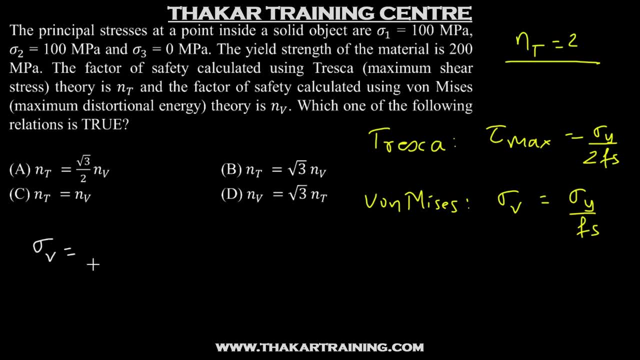 to 2.. The Von Mises stress is given by: And so, substituting the values, we'll have: The first term, sigma 1 minus sigma 2, will be 0.. The second term, sigma 2 minus sigma 3, will be 100 square. 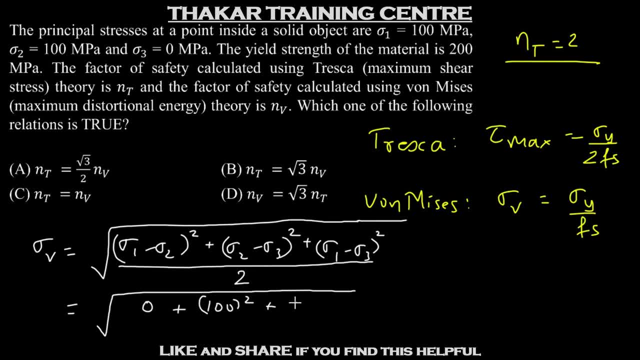 The third term, sigma 1 minus sigma 3, will also be 100 square upon 2.. So we have 2 times 100 square divided by 2.. So 2 and 2 will get cancelled, And then sigma v will be 100 MPa. 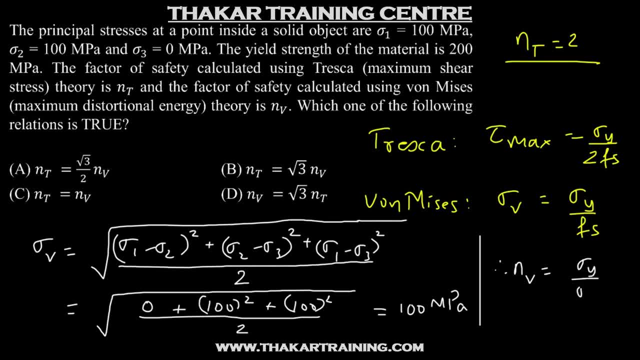 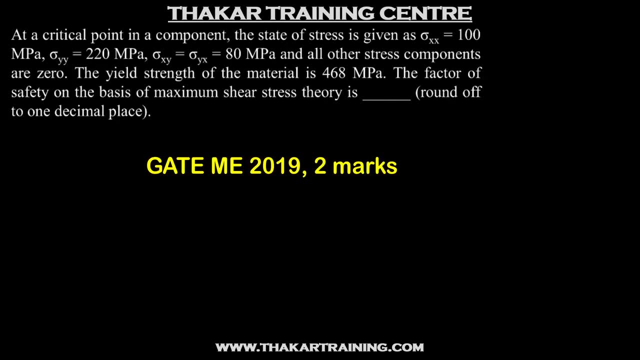 And so Nv will be sigma y by sigma v. That will be 200 by 100, which is equal to 2. So we get Nv is also equal to 2.. The answer for this question will be option C. This question says: at a critical point. 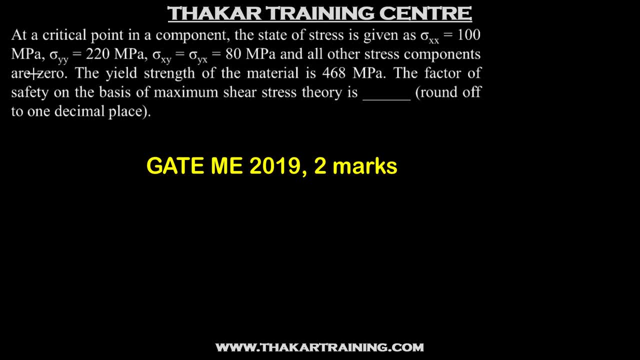 in a component, the state of stress is given as sigma xx is 100 MPa, Sigma yy is 220 MPa And sigma xy, equal to sigma yx, is 80 MPa. All the other stress components are 0.. The yield strength of the material is 468 MPa And we have to find out the factor of safety. 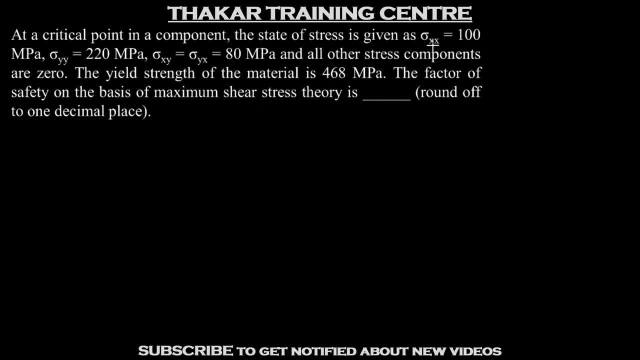 on the basis of maximum shear stress theory. So from the state of stress we realize that it is a plane stress condition. The principal stresses, sigma 1 and sigma 2, will be given by. So these are the usual rotations. Now here, sigma xx means sigma x, Sigma yy means sigma y And sigma xy, equal. 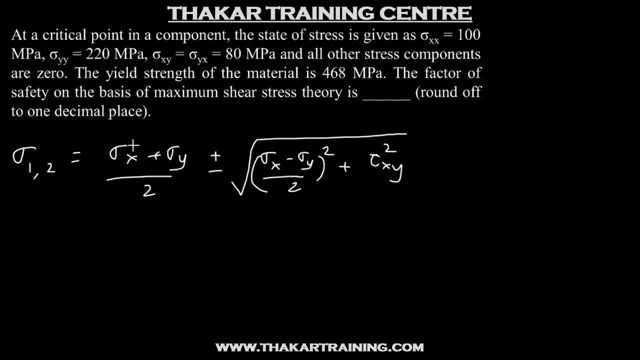 to sigma yx means this is the shear stress tau xy. So let's substitute the values one by one. So, on doing the calculations, we get: sigma 1 will be 260 MPa and sigma 2 will be 60 MPa And since it is plane stress, sigma 3 will be 0. 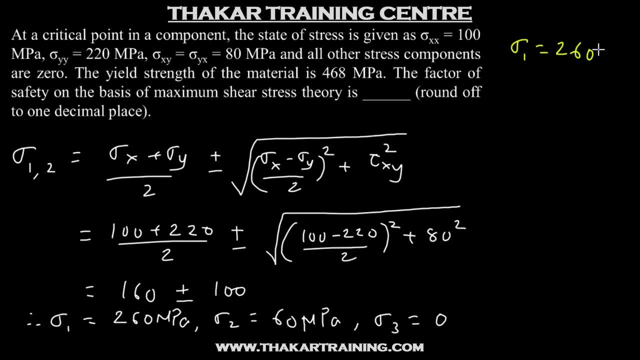 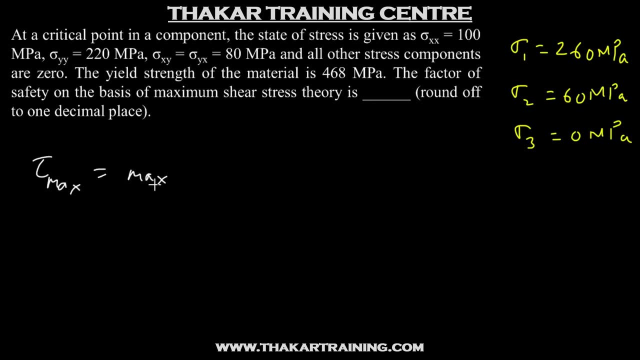 So I will note down the values on the side. Sigma 1 is 260.. Sigma 2 is 60 And sigma 3 is 0.. Now Tao makes will be given by maximum of sigma 1 minus sigma 2 by 2. 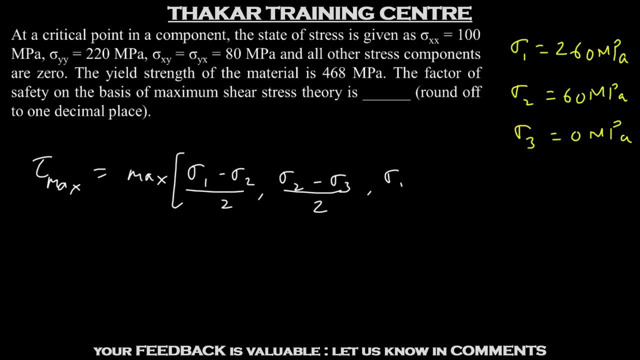 sigma 2 minus sigma 3 by 2 and sigma 1 minus sigma 3 by 2.. So this will be maximum of sigma 2 minus sigma 3 by 2 to a total University. So this will be maximum of sigma 1 minus sigma 2 by 2 to a total University. So this will be maximum of. 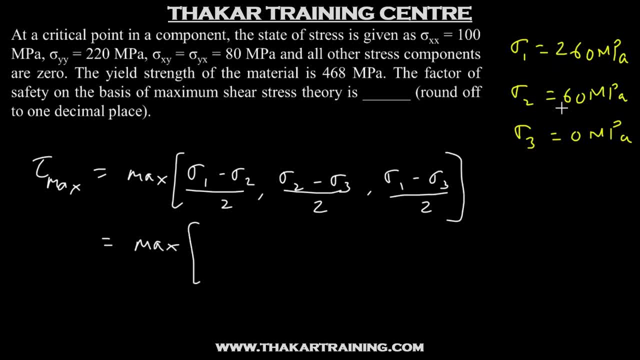 now, sigma 1 is 260, sigma 2 is 60, so this is 200 by 2, this will be 100. sigma 2 is 60, sigma 3 is 0, so this will be 60 by 2: 30 and sigma 1 is 260, sigma 3 is 0, so this will be 260 by 2: 130. so 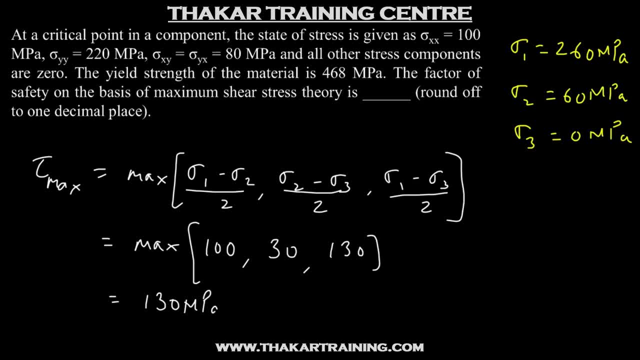 we have: the maximum shear stress is 130, mega pascal. now, by maximum shear stress theory. we have: tau max is sigma y by 2 fs. so the factor of safety will be sigma y by 2 times tau max. so therefore this will be: sigma y is given to us as 468 upon 2 times tau max is 130. 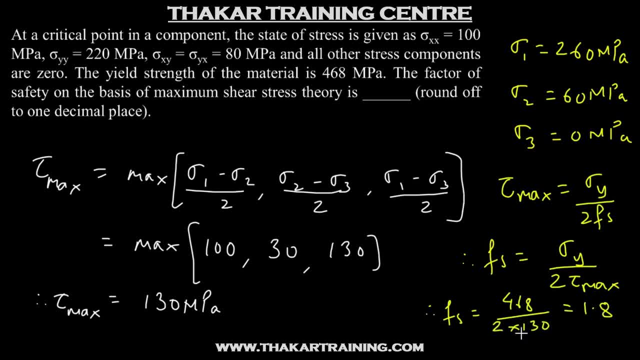 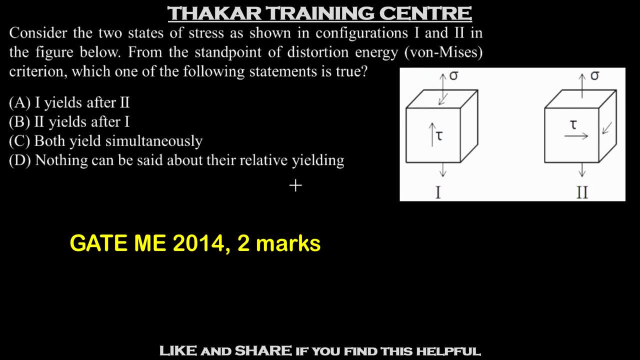 so this on calculation gives 1.8. so the answer for this question will be 1.8. consider the two states of stress as shown in the configurations 1 and 2 in this diagram from the standpoint of distortion energy criterion, that is, the von weiss's criterion. 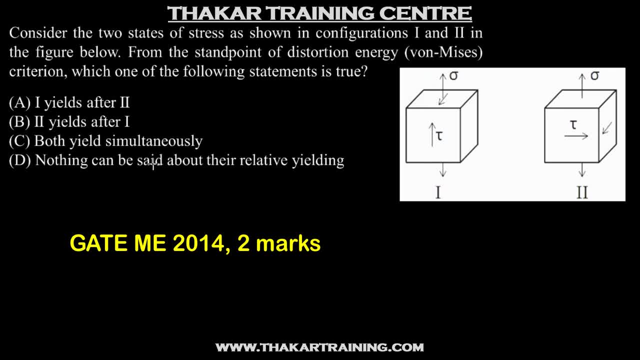 which one of the following statements is true. and these are the options that are given to us now. we are used to writing the von weiss's criterion in terms of the principal stresses, that is, sigma 1, sigma 2 and sigma 3, but in this question they are given the state of stress. 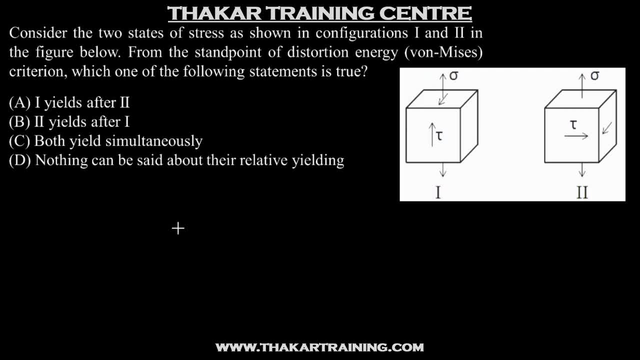 so you can also remember the von weiss's stress in terms of the elements of the state of stress. for questions like these it is given by use this equation. forsay: if the pressure is limited by a corresponds toout theting each sofort of s masses in aerationifie exercised the single surface current, this equation will: 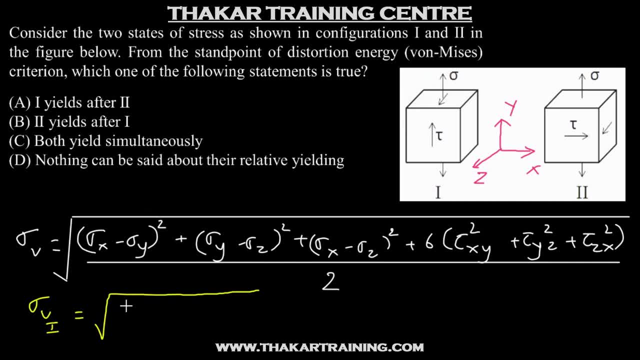 differ. as shown in nytto, find the verse y, F and z direction. so that's why the z direction, and also the first argument, will be 4 of the sigma x and 0 of the x direction. so let's mark a coordinate frame for this question. 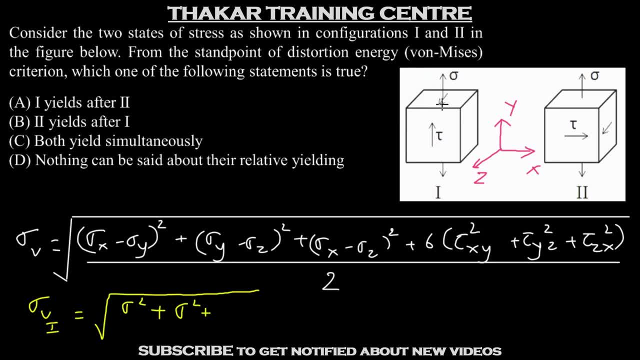 so this x won't make sense. this is y direction and this is z direction. so calculating 1 minus stress will be zero. now, looking at this shear stress, this is tau y z. so we have a 6 tau square term divided by 2, which can be simplified to under root sigma square plus 3 tau square. similarly, 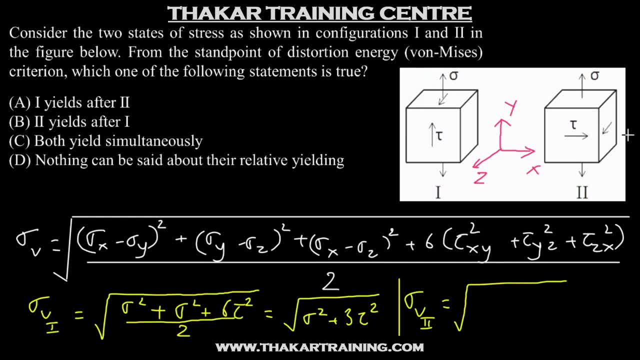 for configuration 2, the von meiser stress will be. so there is no normal stress in x and z direction. so the first two terms will be exactly same: sigma square plus sigma square. this is tau x- z which is given to us. so this will be plus 6 tau square by 2.. so if you see both the 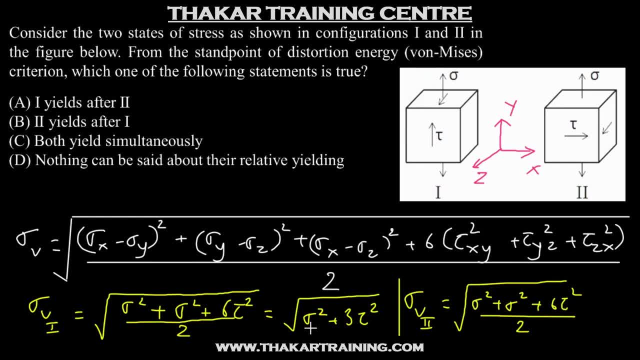 configurations have the same von meiser stress. so even this will be simplified to the same value. that is under root sigma square plus 3 tau square. so what we find is both the configurations have the same von meiser stress. so when they will start yielding, both of them will start yielding together. 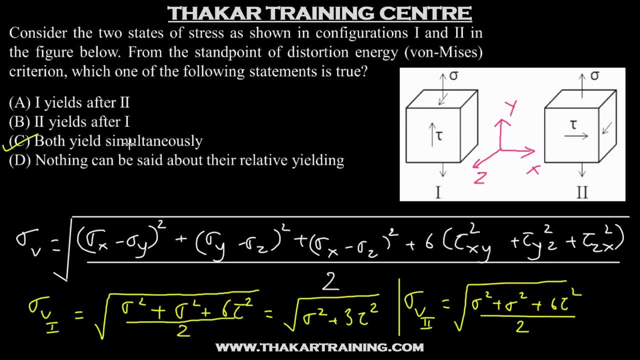 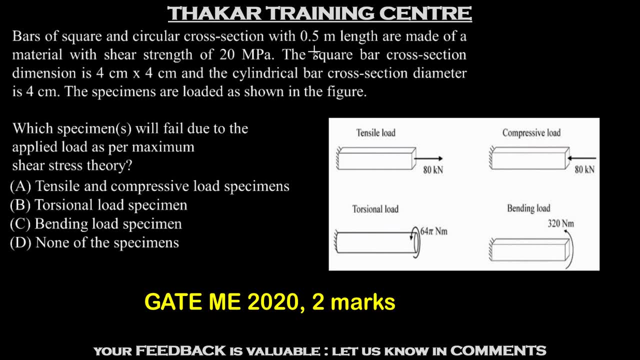 so the answer will be option c. both will yield simultaneously. bars of square and circular cross section with 0.5 meter length are made of a material with shear strength of 20 megapascal. the square bar cross section dimension is 4 centimeter by 4 centimeter and the cylindrical 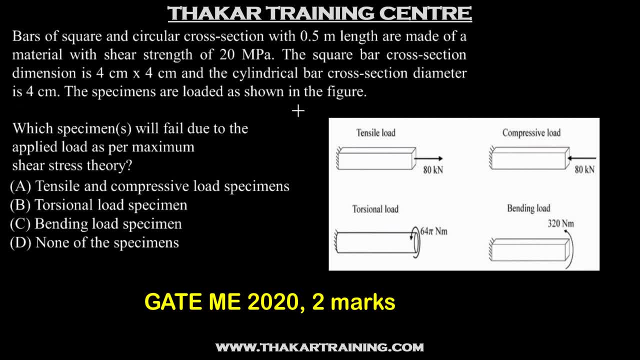 bar cross section diameter is 4 centimeter. the specimens are loaded as shown in the figure. so these are the loadings. which of the specimens will fail due to the applied load as per the maximum shear stress theory? so let's find out maximum shear stress for each of them. 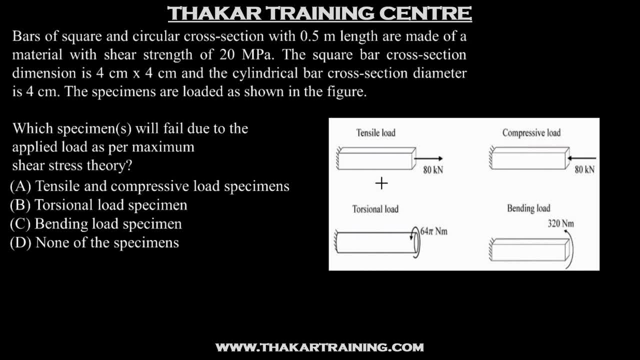 first one is a tensile load. so this is a case of a simple tension. so it will be a uniaxial state of stress. so whatever tensile stress that we will be finding out will be sigma 1 and sigma 2 and sigma 3 will be 0.. so sigma 1 will be the load upon area. 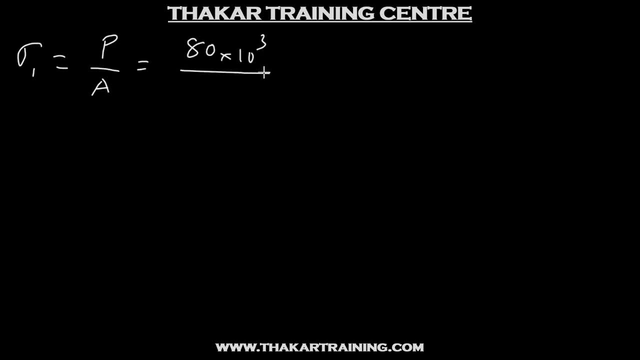 which is 80 kilo newton, so that will be 18 to 10 to 3 upon. this is square bar, which is having a cross section, 4 centimeter by 4 centimeter, so this will be 40 mm by 40 mm, and so this is equal to 50. 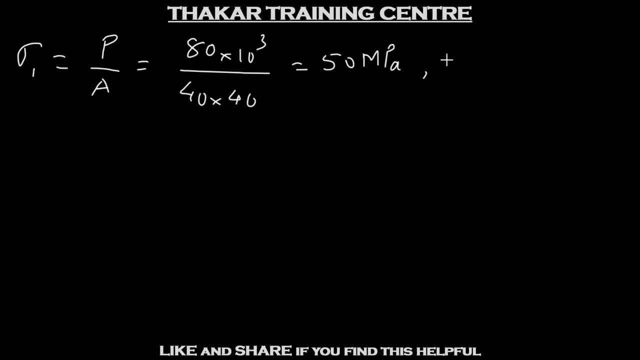 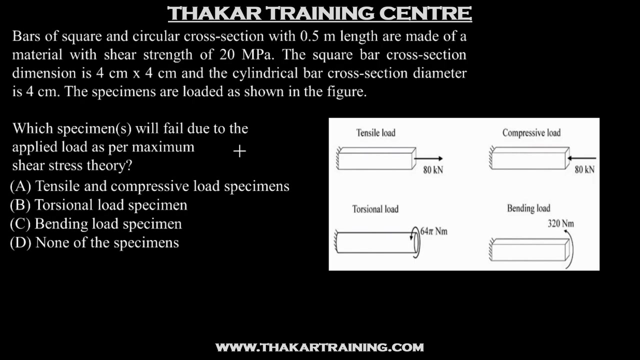 number정이, so logs 0, sigma 1 and sigma 3 are zero. so tau max, which is maximum of sigma 1 minus sigma 2 by 2, and sigma 1 minus sigma 3 by 2 is 25 MPa. So if we look at the question again, the question says the shear strength of the material is: 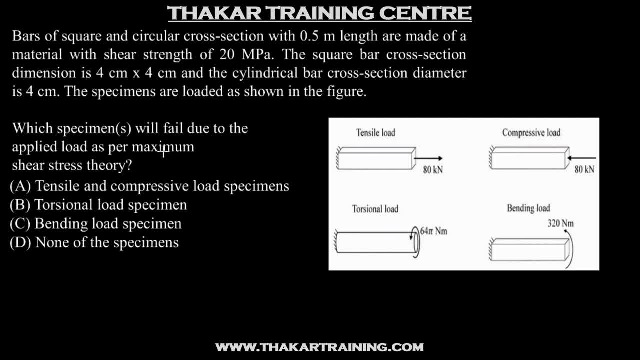 20 MPa and we have to find out which of the specimens will fail as per the maximum shear stress theory. So the options are tensile and compressive load, torsional load, bending load and none of the specimens. Now what we have found out is, when it is a tensile loading case, the maximum shear stress. 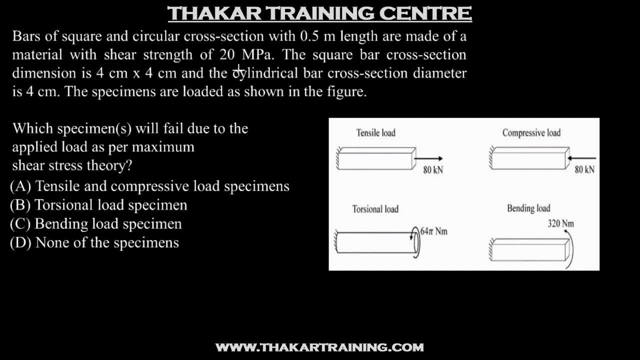 is 25 MPa, which is more than the shear strength of the material. So clearly this tensile load specimen will fail, as per the shear stress theory. So, looking at the options, we do have one of them which will be failing. So none of these is not the answer. and there is tensile load specimen present only in option. 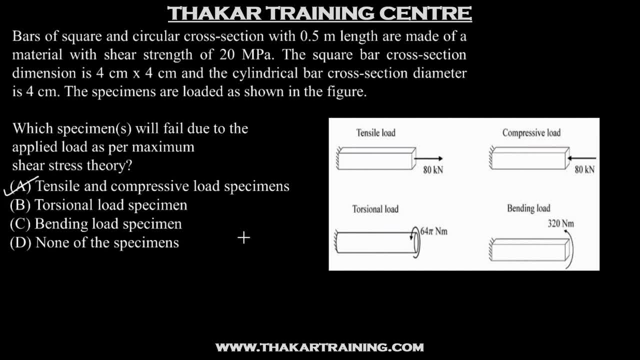 A, So the answer will be option A. So this was asked for two marks. but then when we look at the option simultaneously while solving the question, we figure out that the answer is option A and we do not have to do calculations for all the loadings. 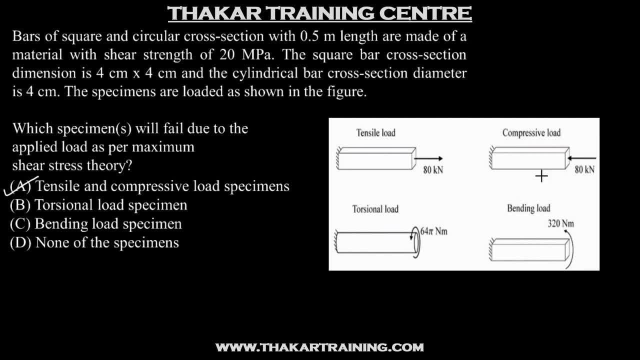 Or you can still go on to verify that. the compressive load specimen will also fail, because in this case what is happening is just the nature of load is changing. So instead of a tensile load specimen we have to do a compressive load specimen. 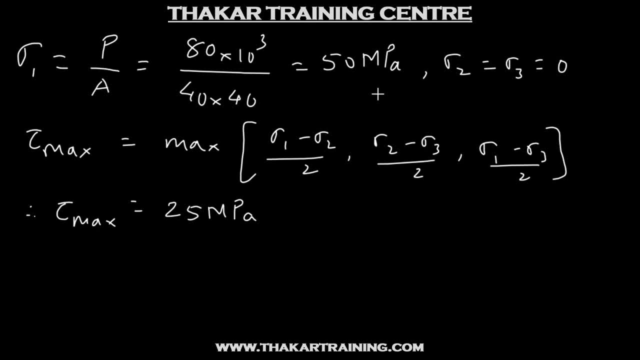 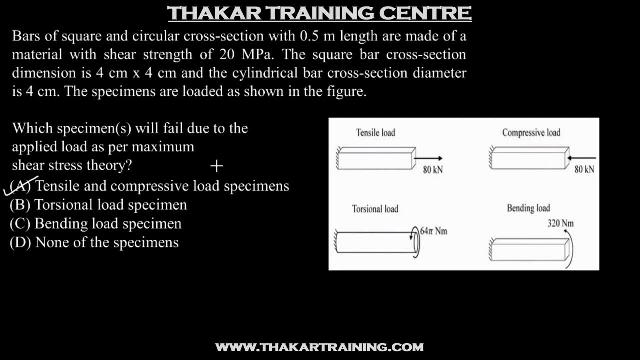 For the tensile load specimen we will have a compressive load specimen of 50 MPa, but then the maximum shear stress will still come out to be 25 MPa, So the compressive loading specimen will also fail, as per the maximum shear stress theory. 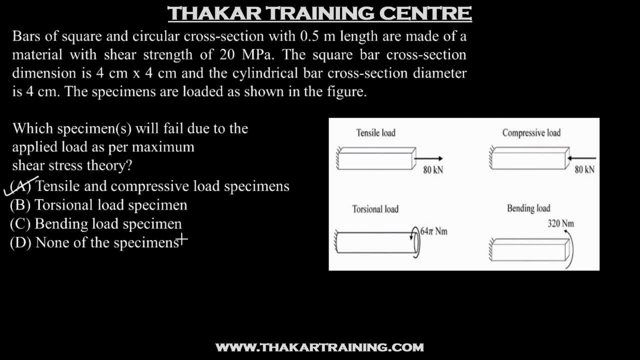 And then you can go on. to verify that the torsional load and bending load specimens will not fail, Their maximum shear stress will turn out to be less than 20 MPa. For this torsional load specimen, we get the maximum shear stress, which is the torsional 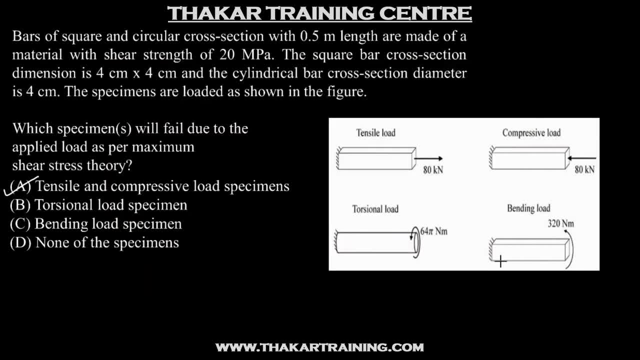 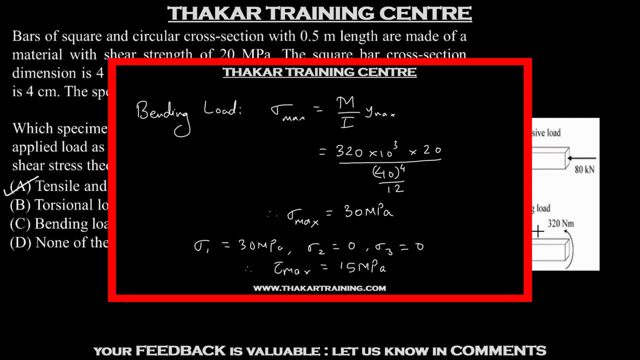 shear stress It turns out to be 16 MPa. and for this bending load specimen we get the maximum bending stress is 30 MPa, Which again is like a uniaxial stress. So the maximum shear stress in that case turns out to be 15 MPa. 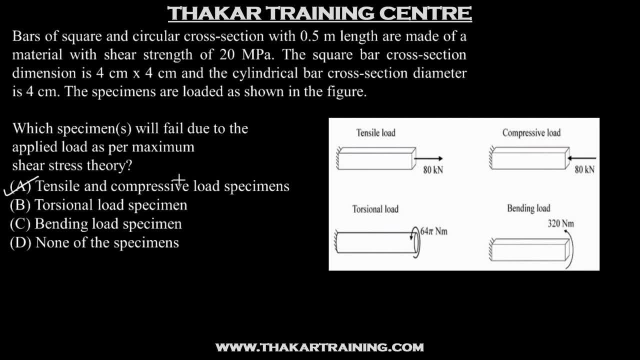 So options B and C do get eliminated and option A is correct, which we actually figured out long time ago. So during a GATE exam, just be alert and just check the options in such type of questions, because otherwise it will take a long time if you first calculate the maximum shear stress. 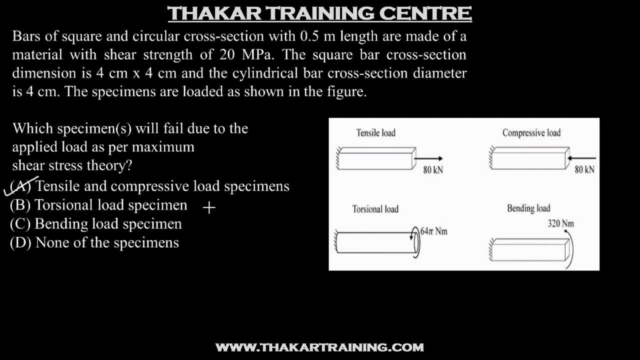 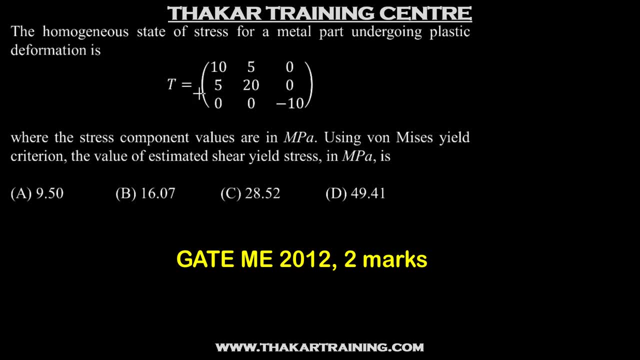 for all the cases and then come to options So you can save time in such questions. The homogenous state of stress for a metal part undergoing plastic deformation is Given by this tensor, So this is a stress tensor. Here the stress component values are in MPa. 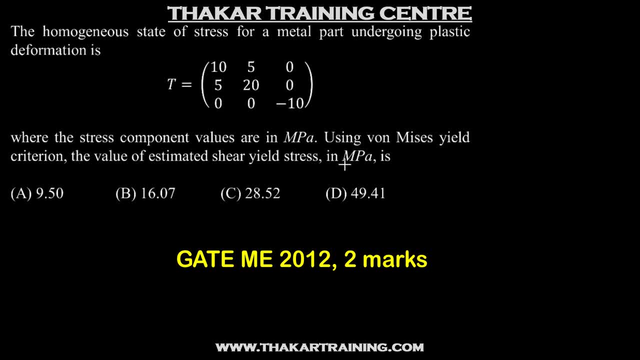 Using Von Mises yield criterion, the value of estimated shear yield strength in MPa is. So what does the question say? That the metal part has started undergoing plastic deformation, So the material has started yielding. So whatever Von Mises stress we get for this state of stress, it will be equal to the yield.